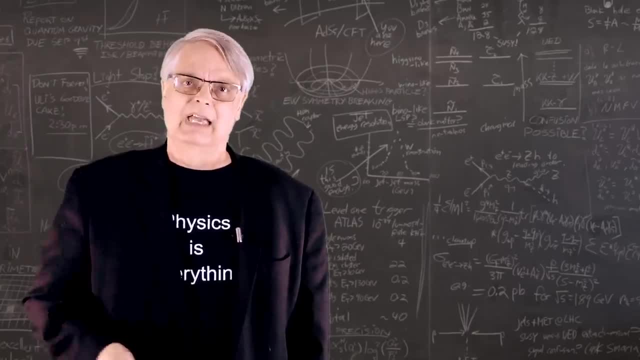 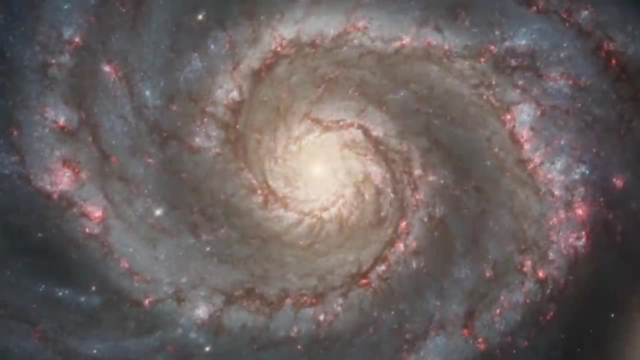 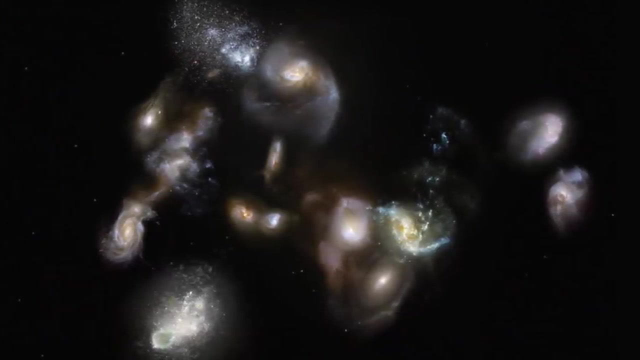 And that's why we believe dark matter exists. Galaxies rotate faster than the observed ordinary matter can explain using the known laws of physics. Ditto with the motion of individual galaxies inside clusters of galaxies And the images of distant galaxies are distorted more than 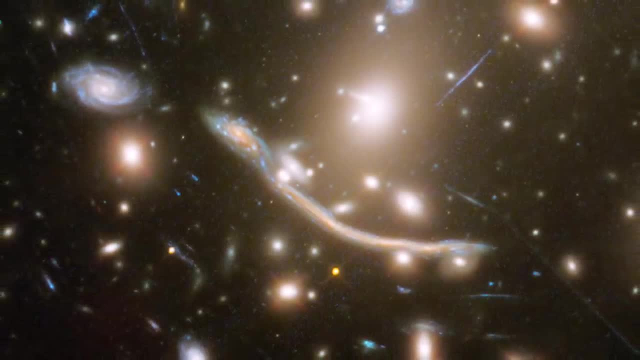 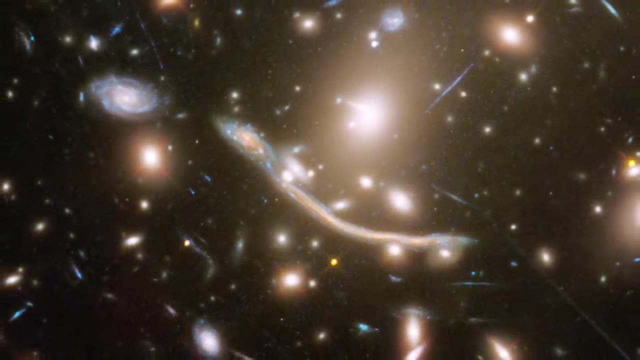 can be explained by the effects of ordinary matter between the distant galaxies and our telescopes. All of these are real, And that's one of the reasons why astronomers believe that dark matter is real. But just what is dark matter? It might surprise you that scientists just simply don't know. 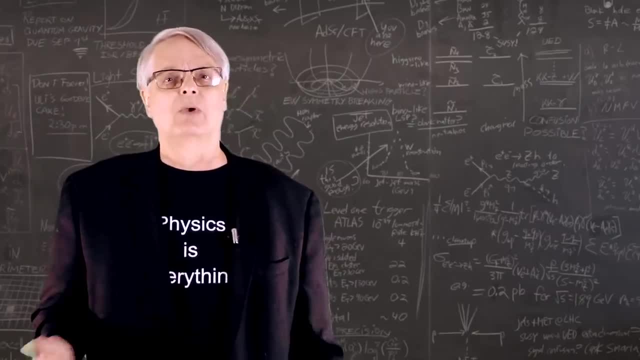 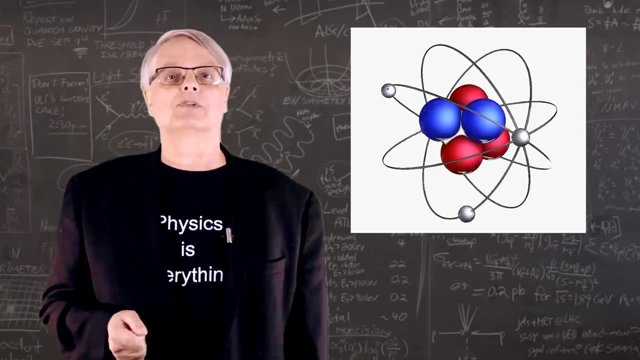 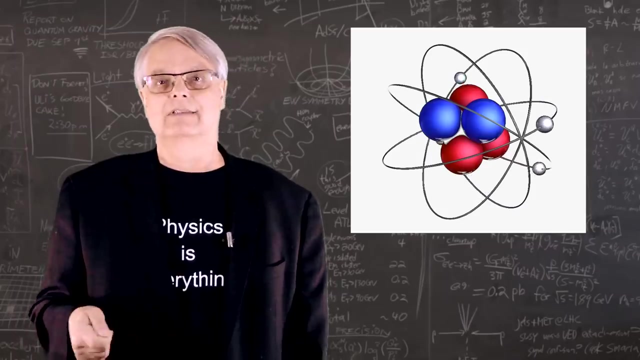 It could be a gas of unknown subatomic particles with a mass much lower than the mass of electrons, or it could be made up of objects as heavy as stars. If you want numbers, the possible range starts with a mass of about 10 to the minus 6 electron volts on the low end, or about 10 to the. 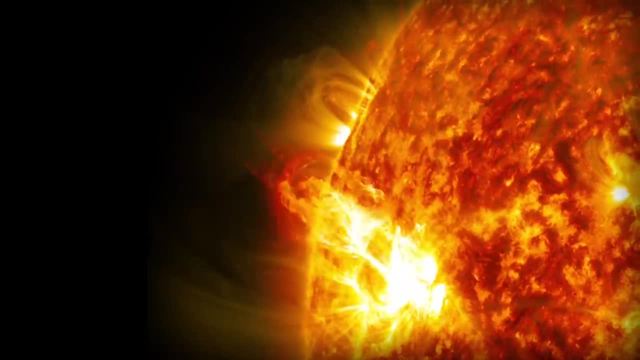 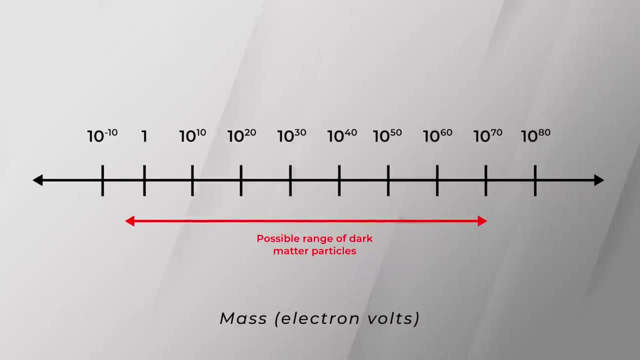 minus 71 solar masses, or about 10 to the minus 7 electron volts on the low end, or about 10 to the solar masses up to a mass of about a thousand solar masses on the high end. That's a ridiculously large range, with the difference from smallest to largest about 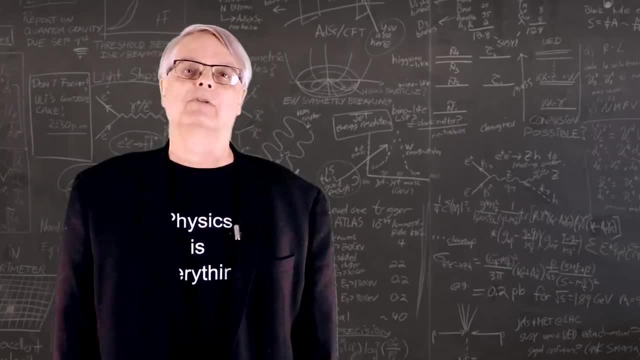 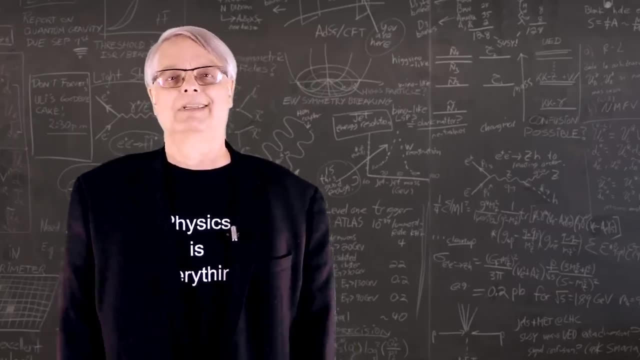 10 to the 75th power. It wouldn't be unreasonable for someone to hear that and conclude that scientists don't have a clue about the mass of individual dark matter particles. That's, of course, not the whole story. After all, scientists have been looking. 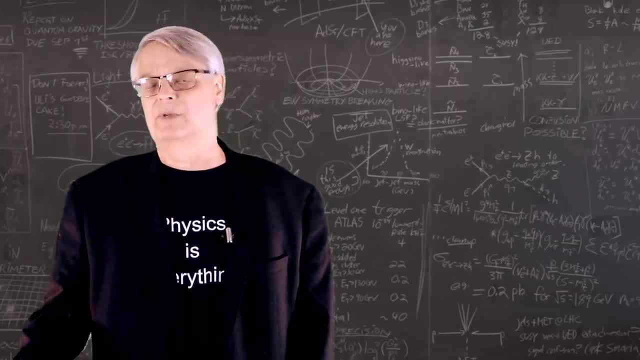 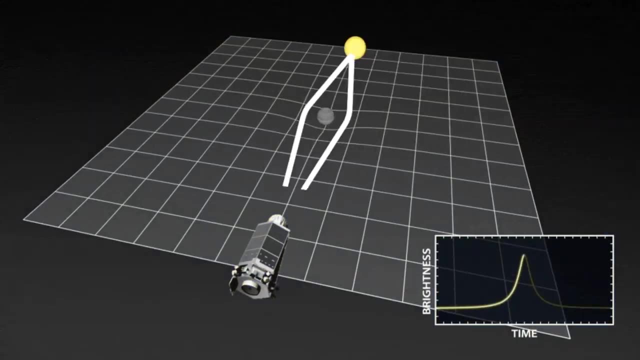 for dark matter for many decades, and some possibilities have been ruled out. For instance, astronomers have used telescopes to look for types of dark matter in the mass range of asteroids, moons, planets and stars. Well, the dark matter can't be seen. After all, it's dark. 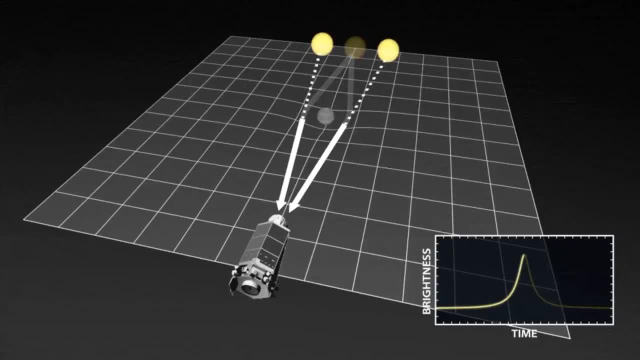 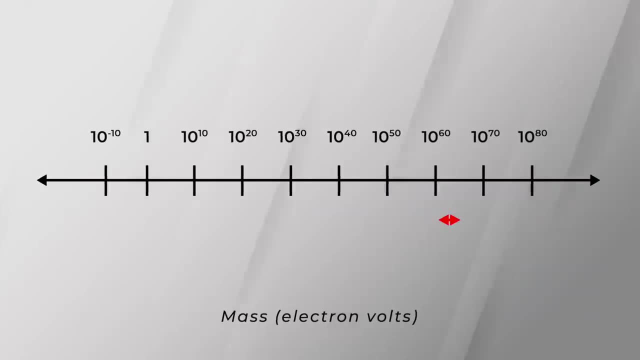 If a dark matter star passes in front of another star, you can detect its passage Using this technique. astronomers ruled out forms of dark matter in the 10 to the minus 7 times the mass of the Sun, to about 30 times the mass of the Sun. That's about the mass of Mercury to 30 solar. 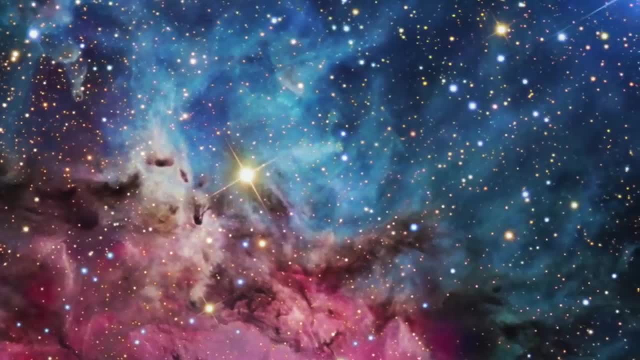 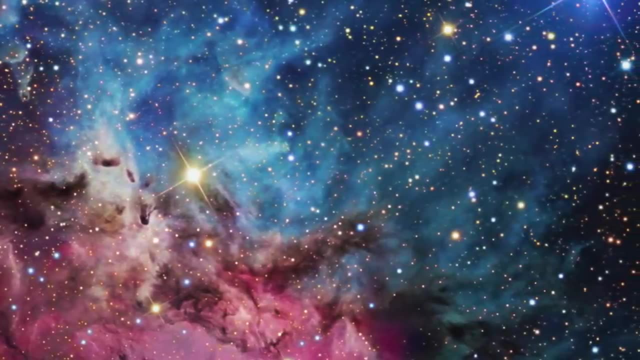 masses give or take. We can actually rule out all candidate forms of dark matter made from non-glowing versions of ordinary matter, like gas, asteroids, planets, etc. simply because they wouldn't be dark, They'd heat up from the light of surrounding stars and emit infrared light. 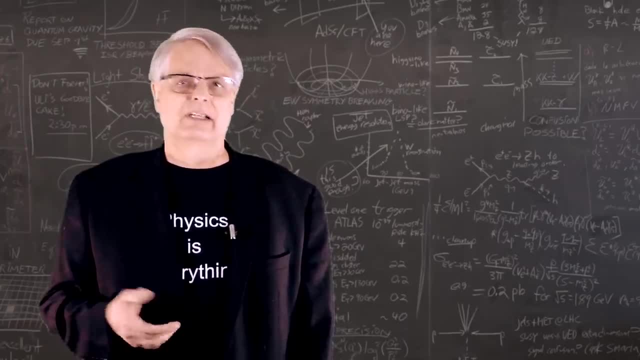 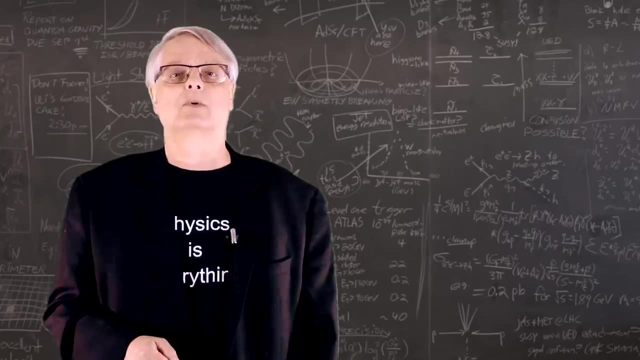 So we can rule out that form of dark matter. Now, for a very long time- most of my career actually- scientists have hypothesized another form of dark matter, what are called WIMPs, short for weakly interacting massive particles. 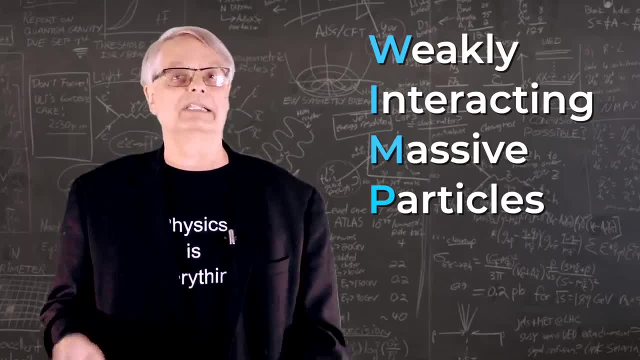 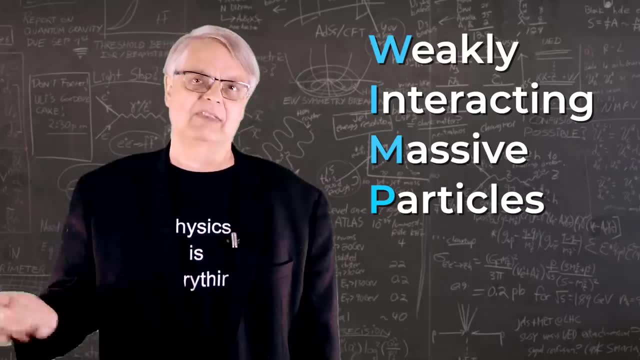 WIMPs are thought to be subatomic particles, kind of like heavy and stable neutrons. The hypothesized mass range was somewhere from slightly lighter than a neutron to maybe 10,000 times heavier, And scientists have looked for versions of this type of possible dark matter. 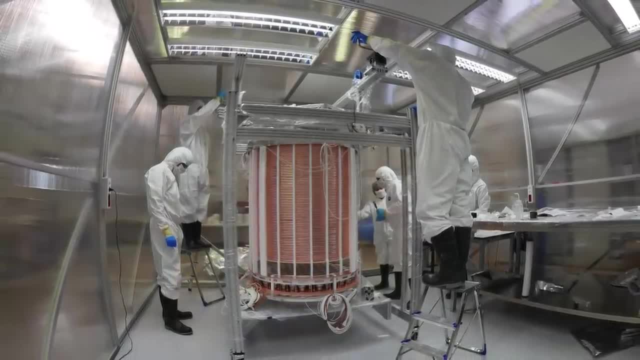 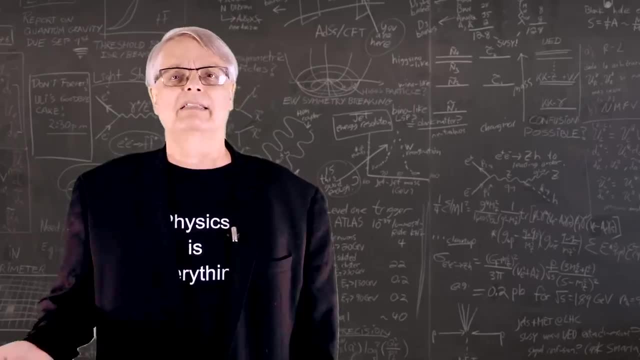 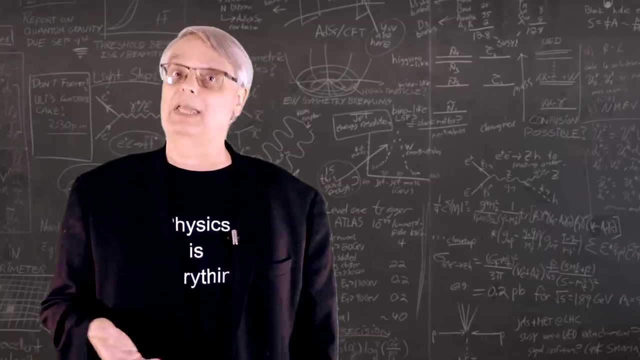 And in spite of decades of looking and huge improvements in detector sensitivity, researchers have found absolutely nothing. Now that doesn't mean that dark matter in this mass range is ruled out, But it does mean that if it exists, it interacts very weakly, maybe only via gravity. 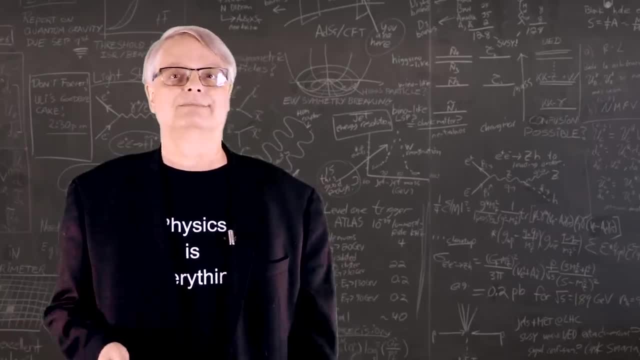 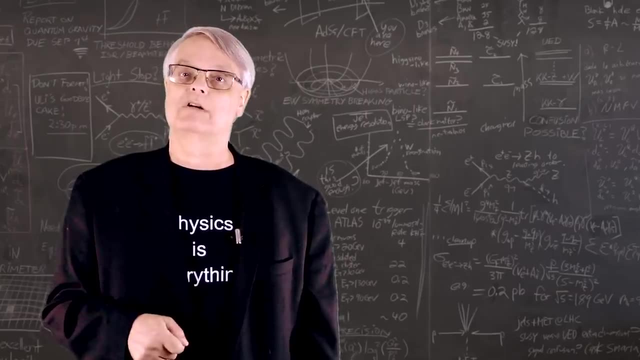 And if dark matter interacts only via gravity, we may never see. However, we really shouldn't be negative yet. Maybe dark matter interacts weakly with ordinary matter, but strongly enough that we can still find it. But that means looking in different places using different techniques. 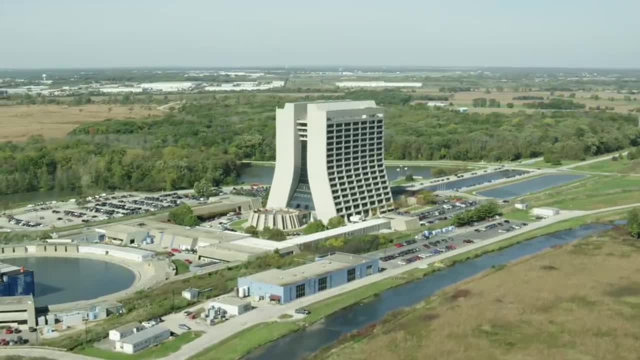 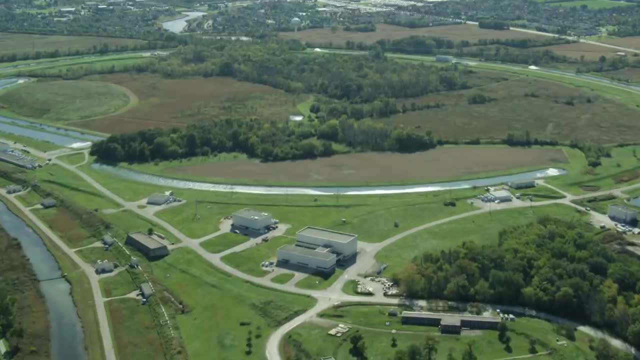 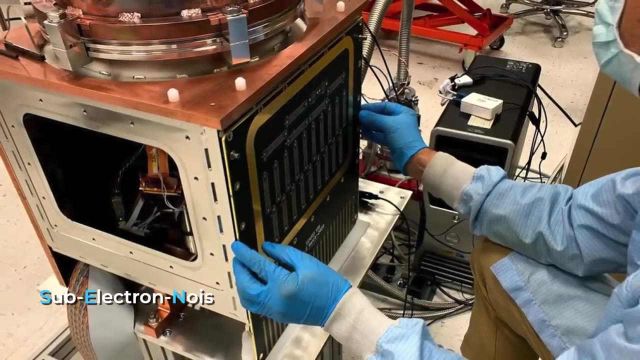 And that's what we're doing at Fermilab in collaboration with a number of sister institutions. Rather than the traditional searches for WIMPs, researchers here are trying different and innovative approaches. Let me tell you about two Sub-electron noise skipper, CCD experimental instrument or SENSEI. 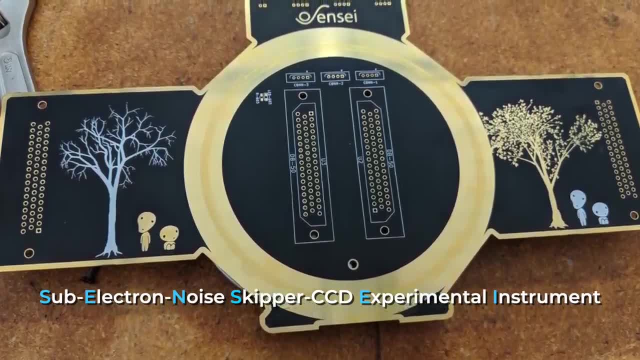 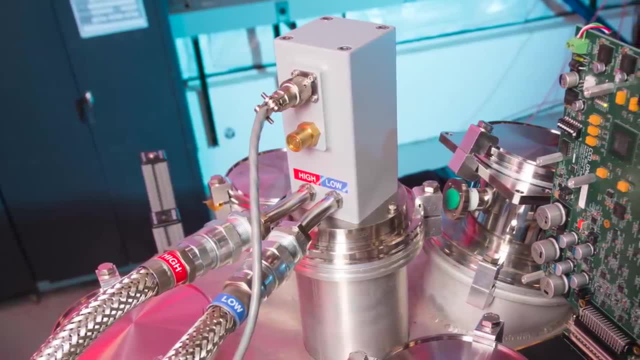 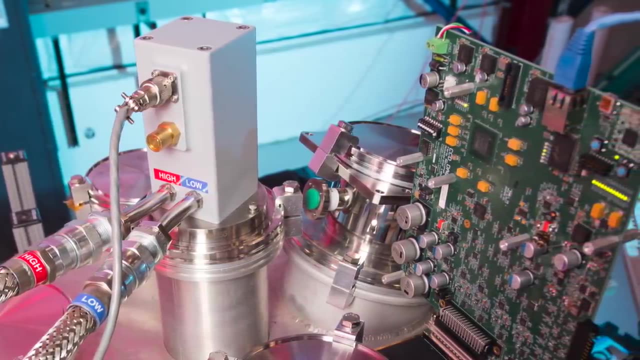 uses ultra-low noise silicon charge couple devices to look for dark matter particles with a mass as low as the mass of an electron, That's 500,000 electron volts if dark matter scatters off electrons in the chip, and as little as a single electron volt if the dark matter gets absorbed by the electrons surrounding the silicon atoms. 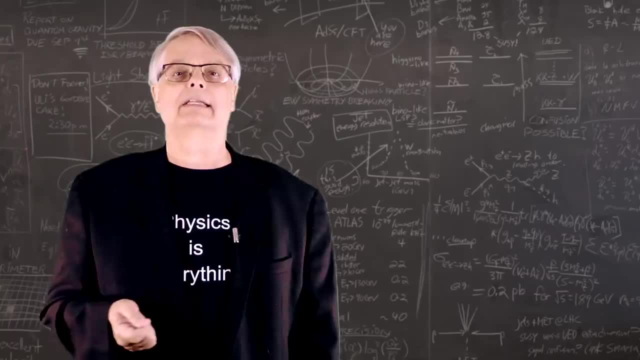 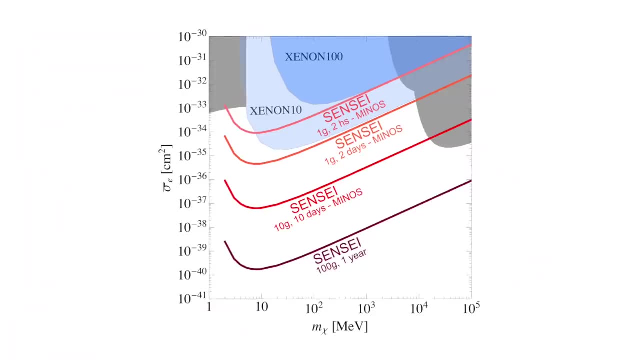 And this isn't just hypothetical. These super-quiet electronic chips are astoundingly powerful for finding low-mass dark matter that interacts with electrons. A single SENSEI detector weighing just 2 grams outperforms a competing detector using liquid xenon. 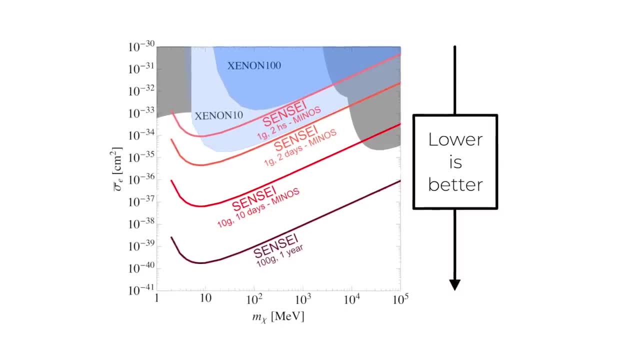 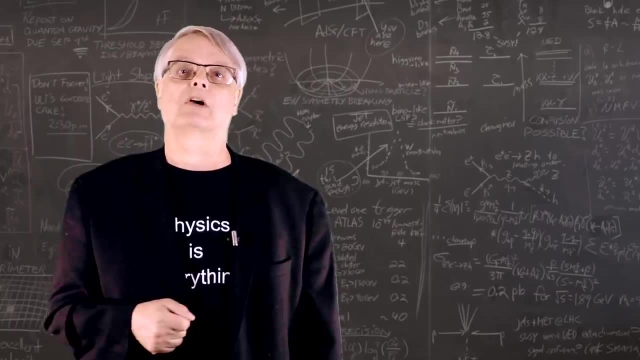 that's a single-sensei detector weighing just 2 grams, outperforms a competing detector using liquid xenon with a mass of a ton, And the SENSEI experiment will be upgraded to a mass of 100 grams. SENSEI is going to totally dominate searches for this form of possible low-mass dark matter. 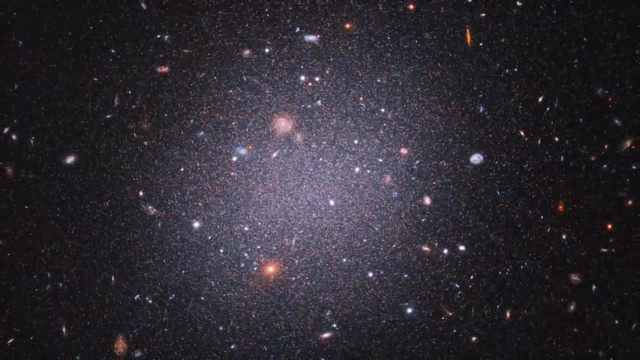 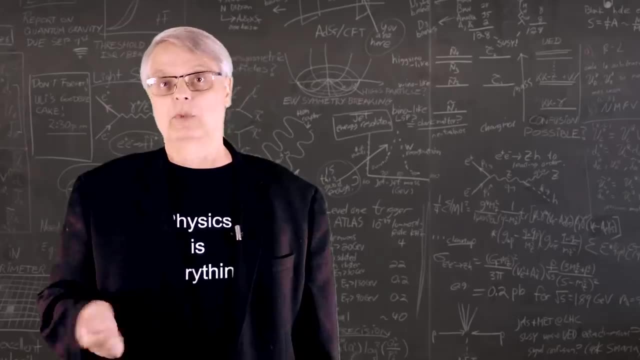 But of course dark matter might not have the properties that SENSEI is designed to detect And given that astronomical measurements have ruled out a lot of very heavy options for dark matter and the WIMP searches have ruled out a lot of possible heavier subatomic particles, 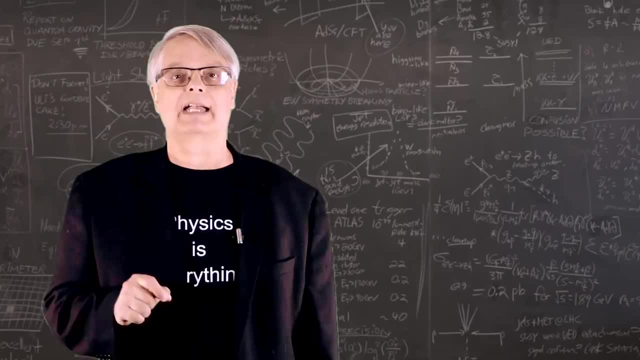 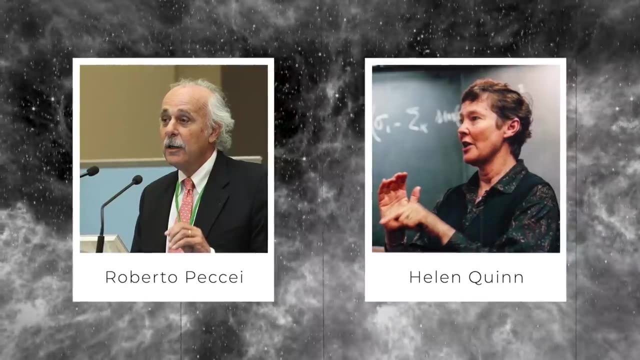 we need to explore more thoroughly the very low-mass dark matter options. In 1977, physicists Roberto Pecce and Helen Quinn were trying to solve a mystery involving the strong nuclear force, According to the theory governing the behavior of quarks and gluons. 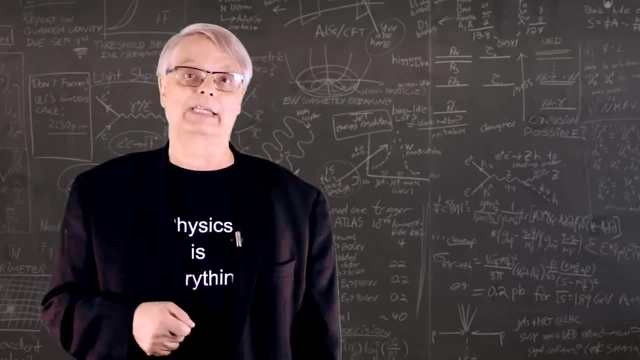 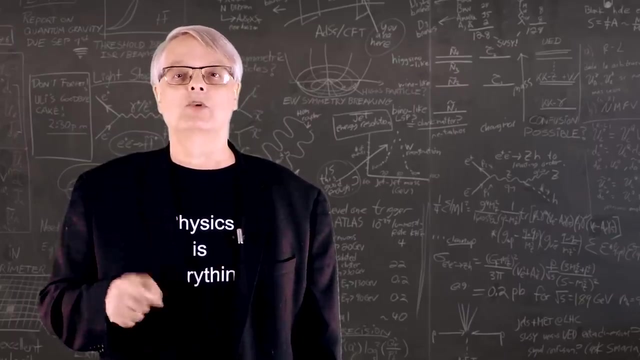 the strong force could favor either matter or antimatter, but it seems to treat both equally. Pecce and Quinn proposed a new energy field that forced the strong force to react equally with matter and antimatter. If that energy field is true, this means that a new particle of energy 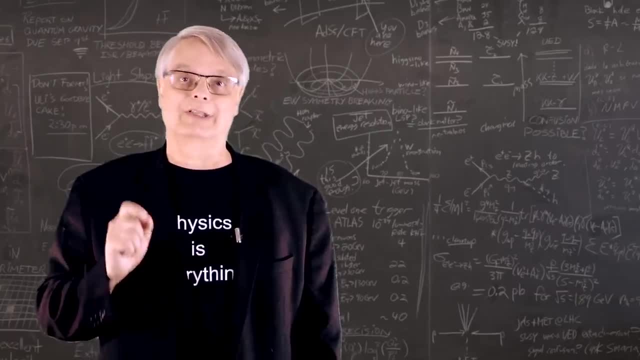 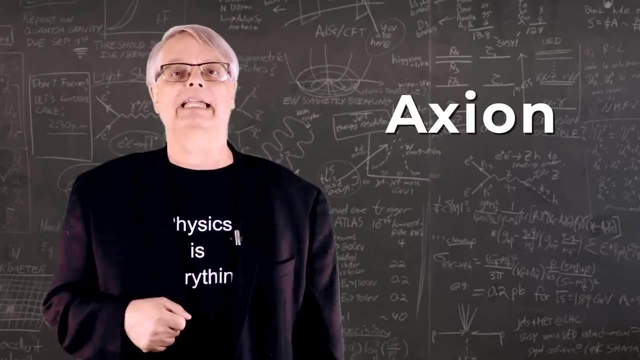 or a particle exists, one that we've never seen before. This particle is called an axion. Axions are very low-mass, don't emit or absorb light and, in short, are a perfect candidate for low-mass dark matter. well, that is, if they exist. 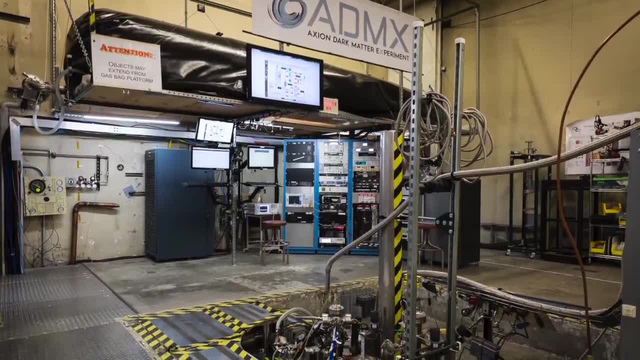 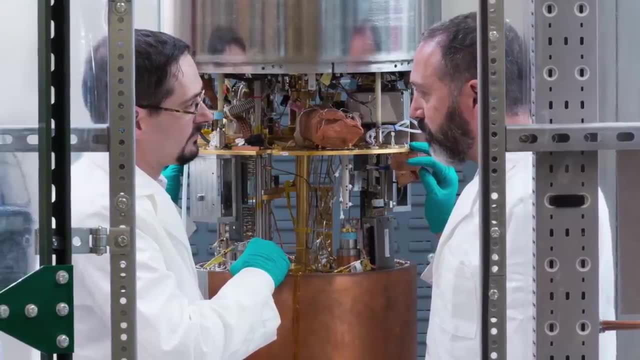 So Fermilab scientists are participating in a collaboration called ADMX, short for Axion Dark Matter Experiment. This experiment uses a very strong magnet and a cavity that resonates at a certain microwave frequency. This experiment uses a very strong magnet and a cavity that resonates at a certain microwave frequency. 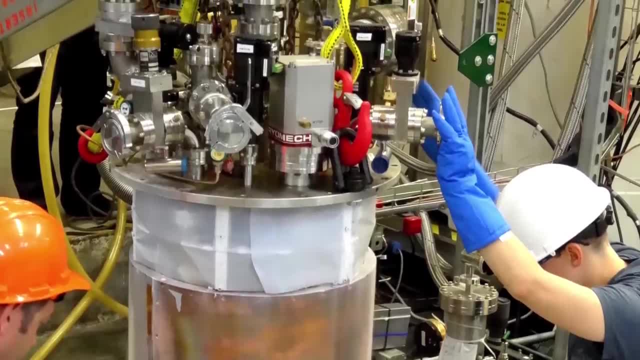 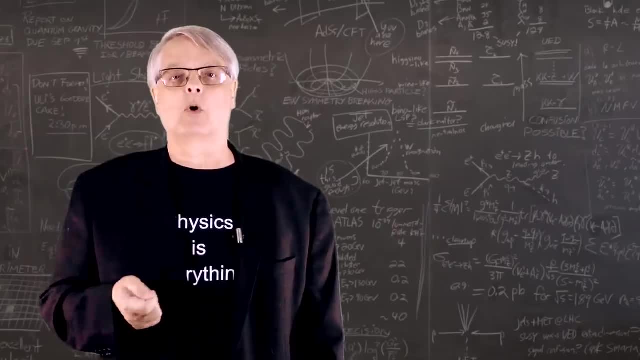 It's a bit like when you blow across the top of a 2-liter bottle and it makes the sound of a specific frequency, Except of course it's microwaves and not sound. The experiment depends on a quirk of axion theory. 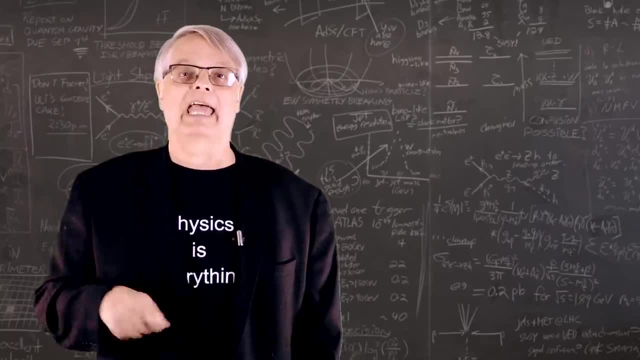 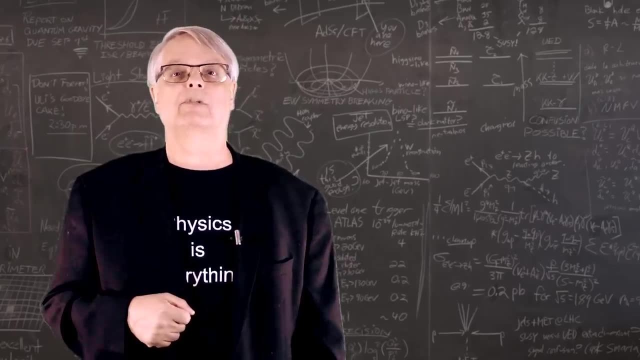 which says that in the presence of a strong magnetic field, an axion can convert into a microwave. It's a tiny effect, but the microwave cavity is surrounded by super-powerful amplifiers that make it possible to see the conversion of an axion to a microwave. 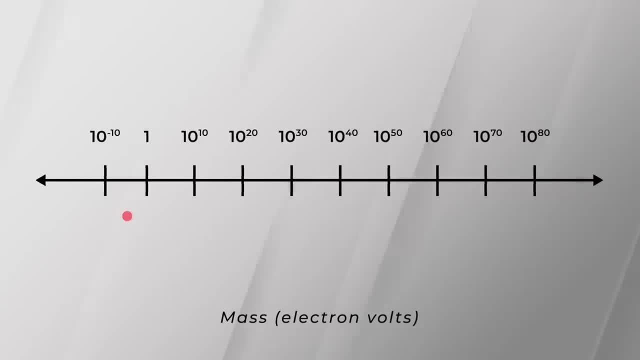 The ADMX experiment is designed to test the ability of the microwave to detect the reaction of an axion. The experiment is designed to look for axions with a mass of about 3 millionths of an electron volt. This is at the bottom end of what scientists think is reasonable for dark matter.